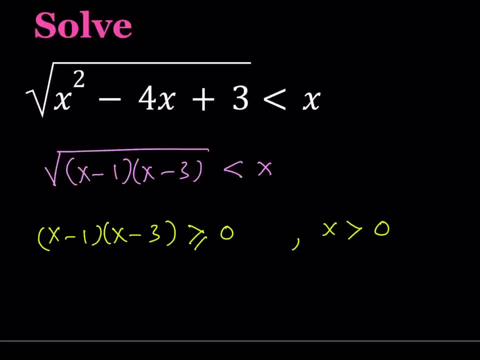 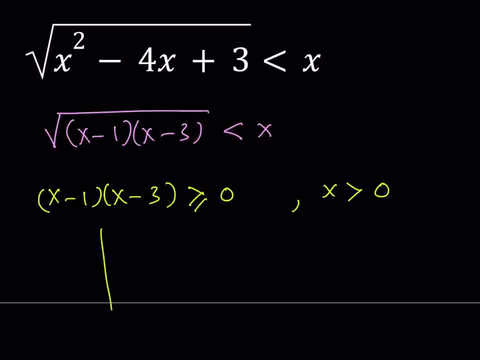 also needs to be positive. Great, So we have two conditions. We're going to be solving those first. but this doesn't solve the inequality, it just gives us some information about the domain. All right, so to solve this, we can kind of put all this together in one table. So I do want 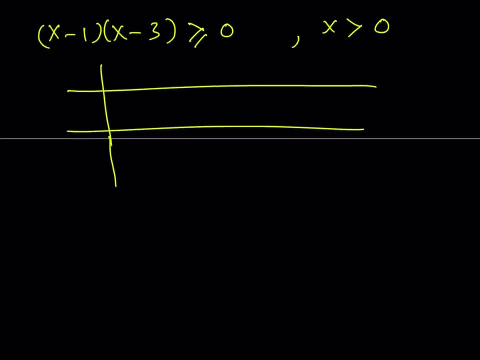 I do want something like this. Let's see, I do want. I'm going to be using 0 as a root, 1 and 3.. This is going to be my first expression, which is x minus 1 times x minus 3.. And this is: 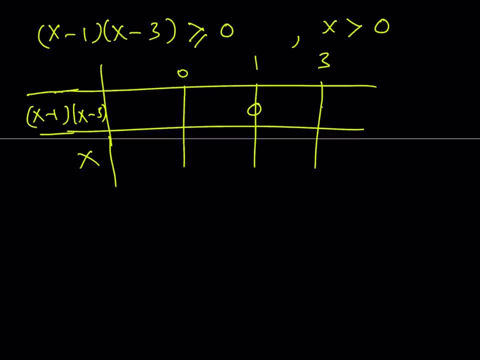 going to be the x. Now, I do have two roots here and one root here, And using the method of intervals, I know that 3 to infinity this is positive, negative and then positive. If x is positive, this is positive and otherwise negative. Great, So here's what I want. I want the intersection. The top is going to be: 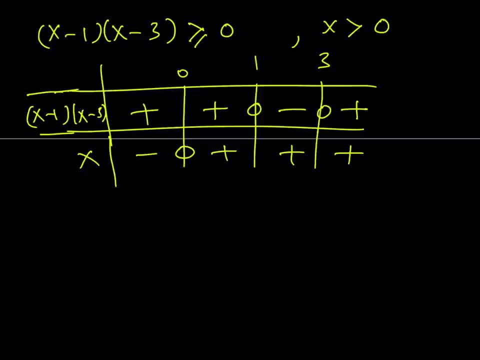 positive and the bottom is going to be positive as well. So I'm looking for the plus plus. So here's my domain. My domain is going to be this interval and this interval. Okay, So that means x needs to be between 0 and 1 or greater than. 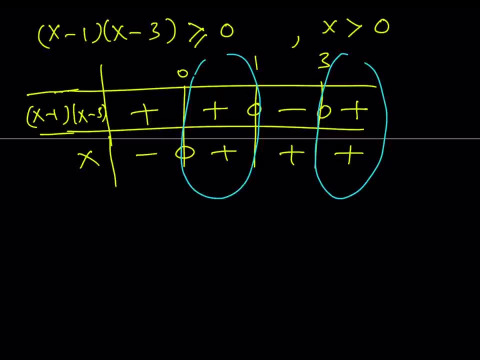 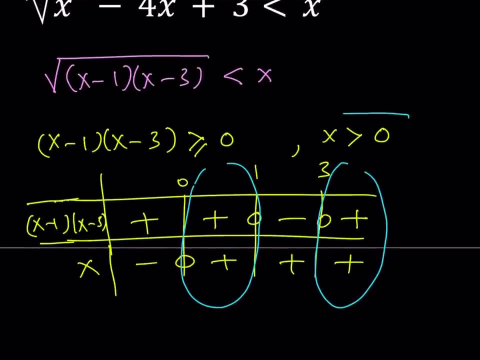 3.. But let's see if any of those numbers will be included. So this gives me the interval 0 to 1.. So is 0 included. Let's take a look at it. x cannot equal 0.. x needs to be greater than 0. So 0 is not. 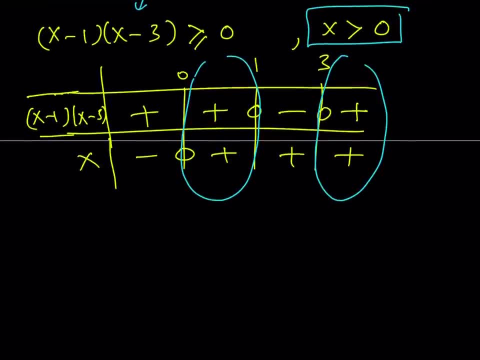 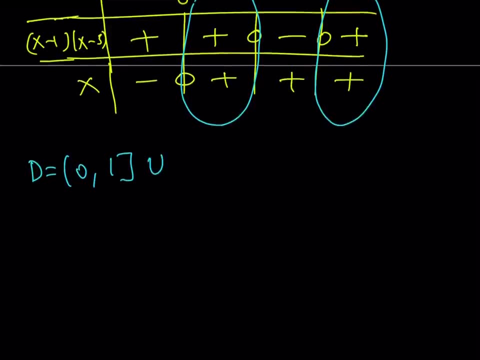 included, but 1 is included because of this. So I'm going to write it like this: 0 to 1, half closed interval and then union- This is my domain, by the way- Union 3 to infinity, But 3 is included, so I. 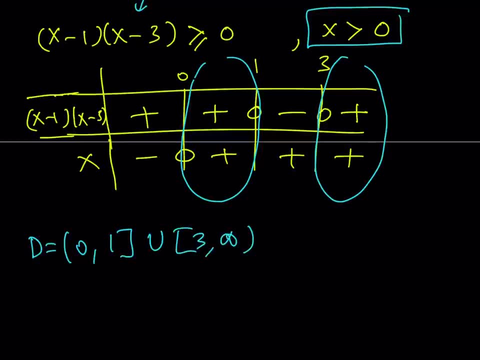 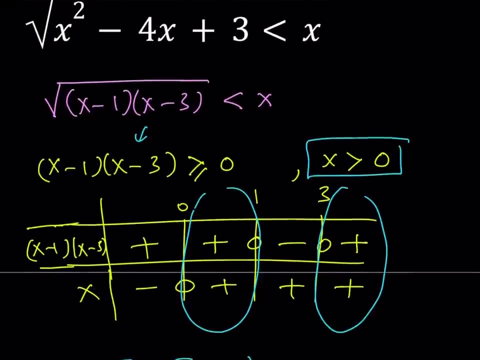 can include it, but infinity is never included. Great. So that's my domain. When I solve inequality, I have to pay attention to the domain. Now let's go ahead and talk about solving this inequality. I'm going to rewrite it in the original form. 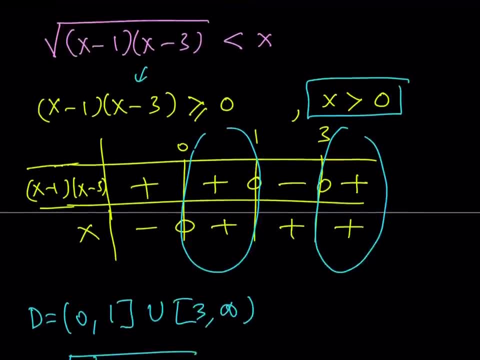 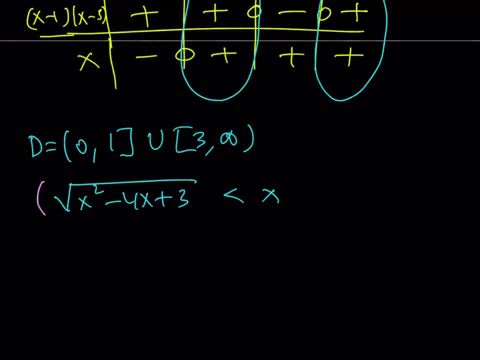 to solve it because I already checked the domain, so I'm good with that. This needs to be less than x. Let's go ahead and square both sides. Obviously, squaring brings some problems, but not when you check the domain. Hopefully you're not going to get extraneous solutions from here, So when you. 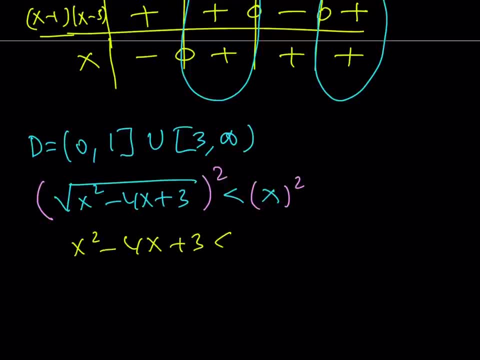 square both sides, you get this basic thing: x squared cancels out. That's why we kind of square both sides and we can put the 4x on the right hand side and leave the 3 on the left hand side and then flip sides, So it. 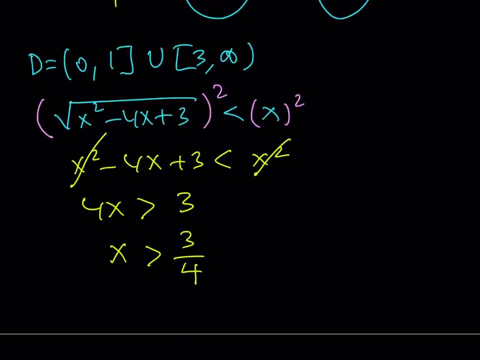 looks like this, and this gives you: x is greater than 3 fourths. So this is the solution to my inequality, but this needs to be consistent with the domain, because if my solutions are not within the domain, then we have a problem. Okay, So I got to make sure that x is greater than 3.. So I got to 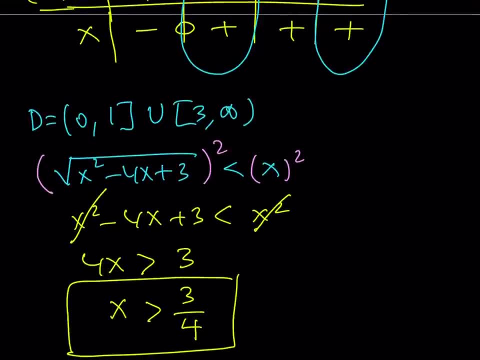 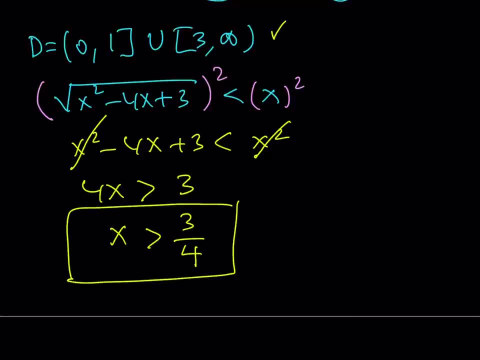 is allowable. Let's go ahead and check here. Well, my domain says something like this. right, So my atac values needs to be between 0 and 1, or 3 to infinity. Well, if you check 3 forths here, If x is. 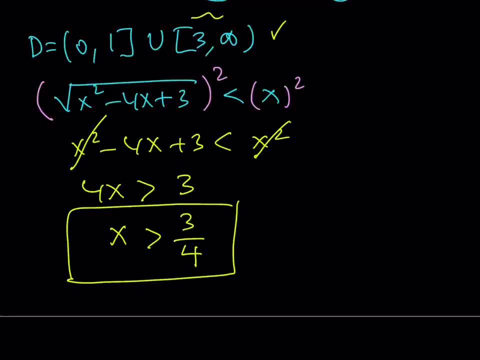 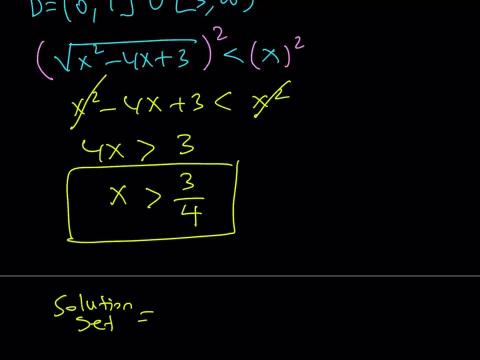 greater than 3 fourths. this part is okay, but this part is not completely okay. Why Be have to cut it at 3 fourths? So my solution set, then, is going to look like this. My solution said x is greater set. the solution set is going to be made up of all the x values, such that x is between three. 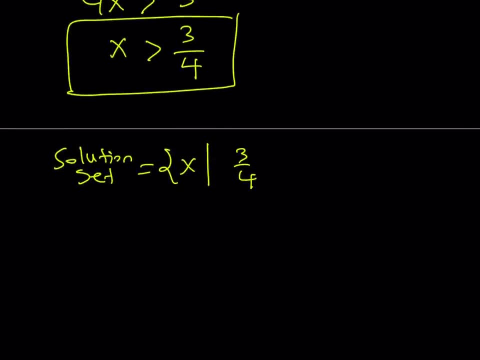 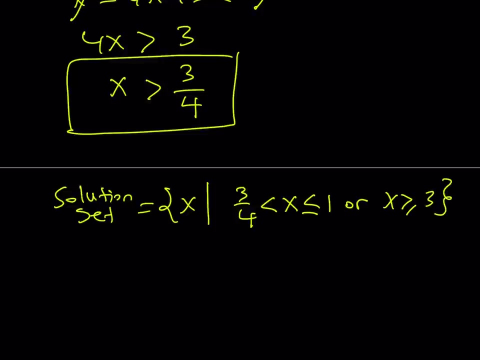 fourths and one. okay, so i'm going to write it like this: x is between three fourths and one, and remember one was included, so i'm going to include the one, or x is going to be greater than or equal to three. why did we have to cut it like this? because the solution does not completely overlap. 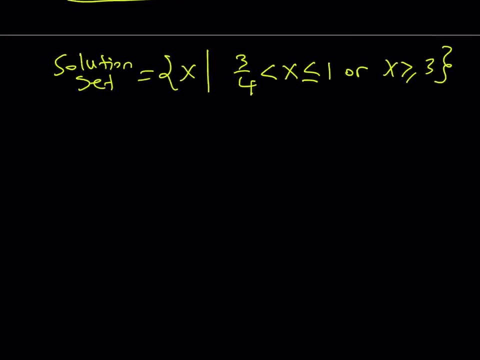 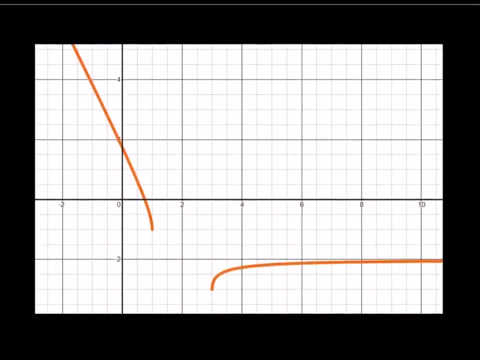 with the domain of the function. and this brings us to the end of this video. well, thank you for watching. i hope you enjoyed it. well, actually, this doesn't bring us to the end of this video because i wanted to show you something, and that is: i almost forgot to graph of this function what 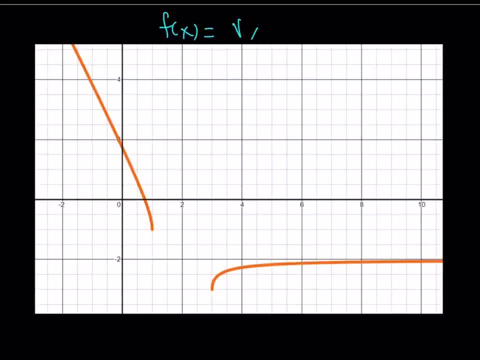 function. well, i kind of graphed the square root of you, x squared minus four, x plus three minus x, and remember that we were saying that this needs to be less than zero because x was on the other side. and what are you looking for? well, basically, you're.